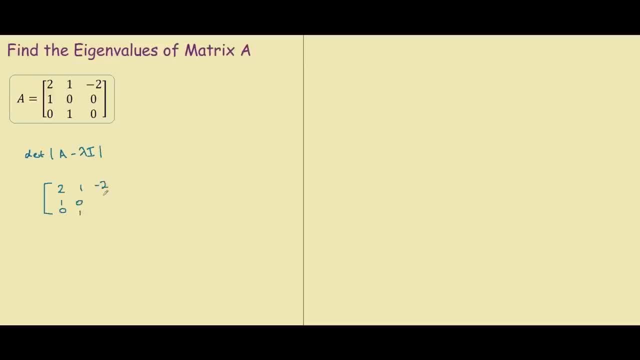 minus pi lambda times the identity matrix, which is 1 0 0 0. 1 0 0 0, 1.. And when we simplify this down, we have 2 minus pi lambda. 1 minus pi 0 is 1, negative 2, 1, 0 minus pi lambda is negative lambda. 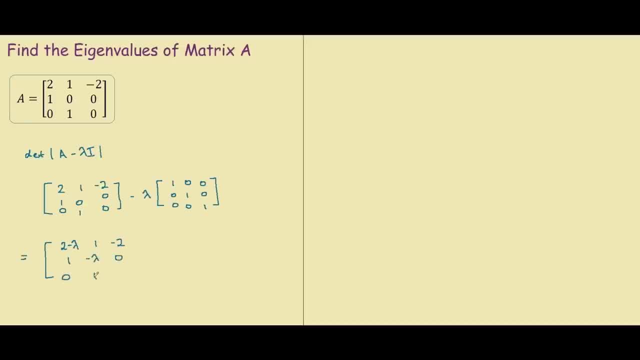 0, 0, 1 and negative lambda. So now our next step is to find the determinant of this three by three matrix. So, if you guys remember, how to find the determinant is, we look at this term here, 2 minus lambda, and then we ignore the rows and columns for this term and look at these four: So negative lambda. 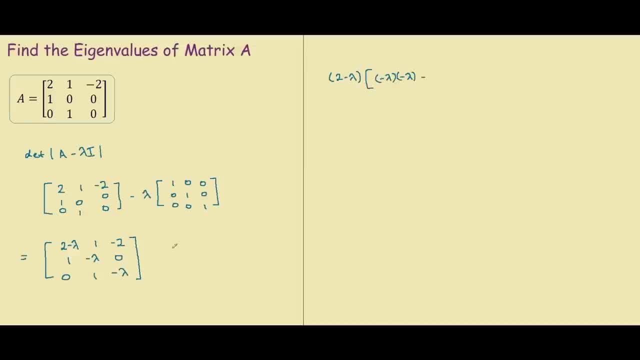 times negative lambda minus pi: 0 times 1.. So that's how you find the determinant of a two by two matrix. If we focus on this section over here, Our next step is to minus 1.. So we minus this term over here. 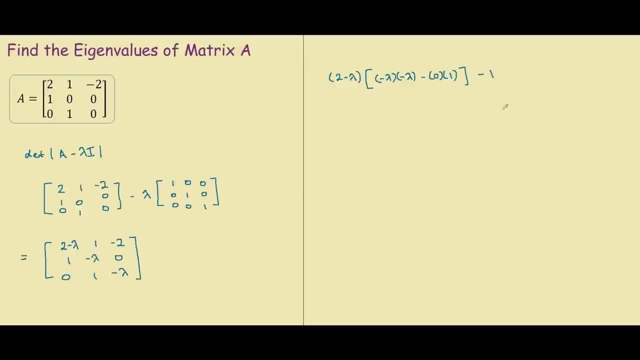 and we focus on the 1, 0, 0 negative lambda. So we have 1 times negative lambda is negative lambda minus pi 0 times 0. Which is 0. And then we plus the negative 2 term, So plus negative 2 times the determinant. 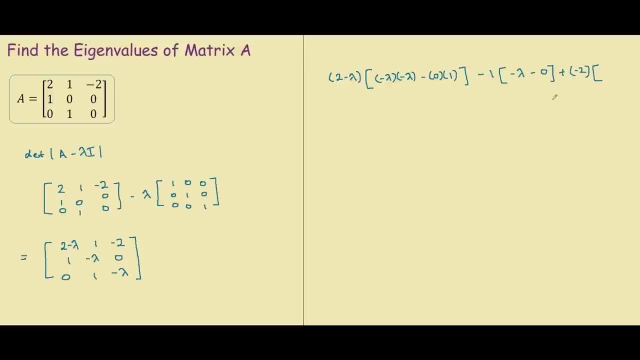 of 1, 1 negative lambda 0. So that would give us 1 minus pi 0.. So this is the determinant of A minus lambda i, And if we simplify this down, we have 2 minus lambda. Inside the square brackets we only have lambda squared. 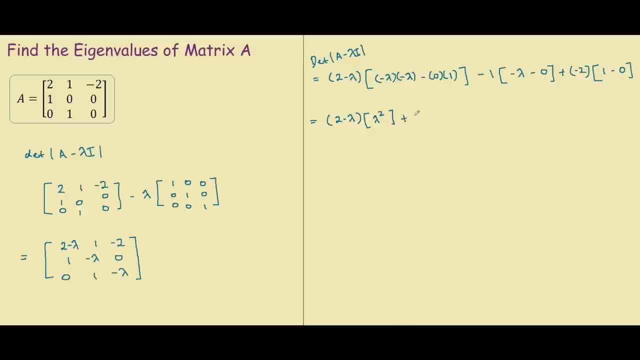 Minus pi 1 times negative lambda is plus lambda, And then plus negative 2 times 1 is negative 2.. So, after finding the determinant, what you want to do is make this equal to 0. So basically saying this equals 0. So that we can solve for lambda.